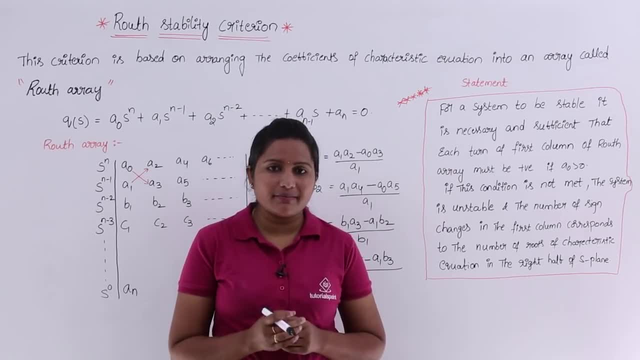 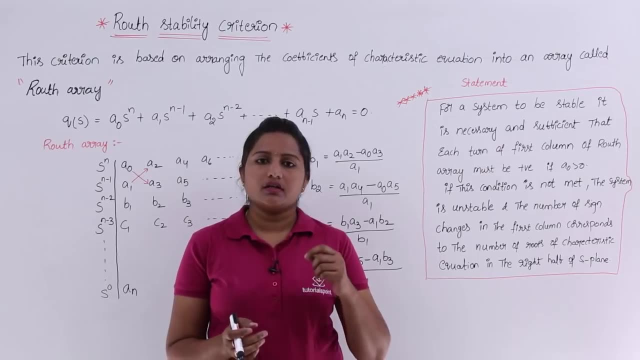 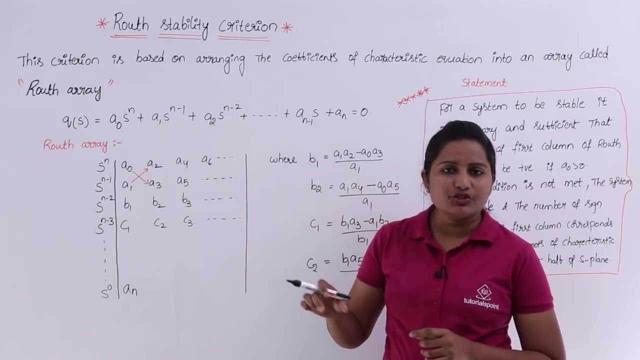 In this video we are going to discuss about Routh Stability Criterion, which we already discussed, that this Routh Stability Criterion is used to calculate the stability of the system. So here you can see. this criteria is based on the arranging the coefficients of a characteristic equation in the form of array. that array is also called as Routh. 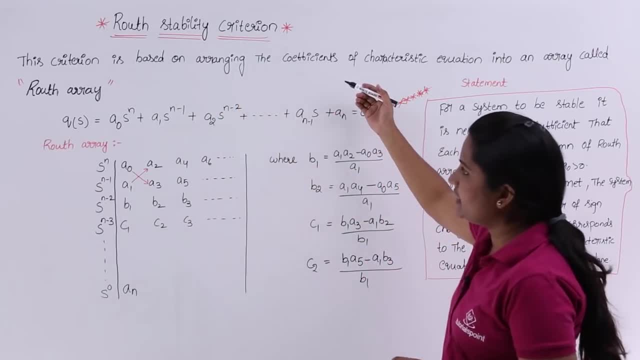 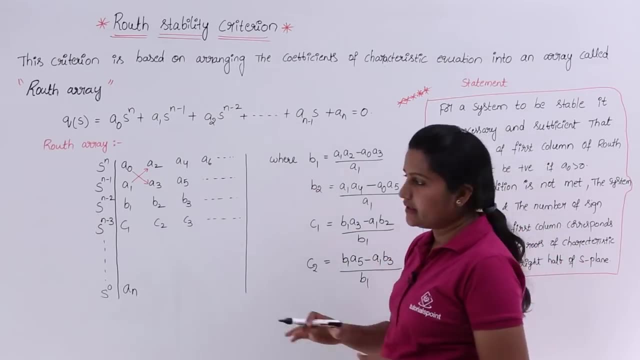 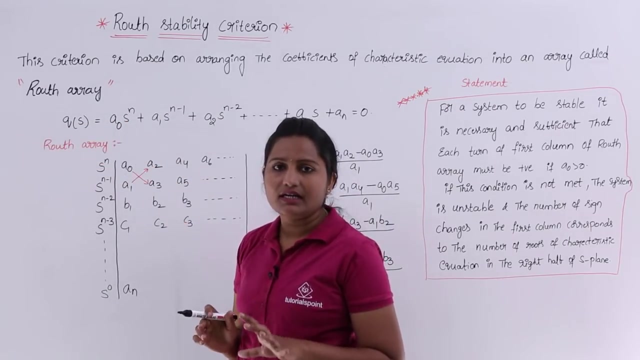 Array. So you can once again see the definition. this criterion is based on arranging the coefficients of characteristic equation in an array, is also called as Routh Array. For example, if your characteristic equation is in this form, so Q of s, I am considering that as my characteristic. 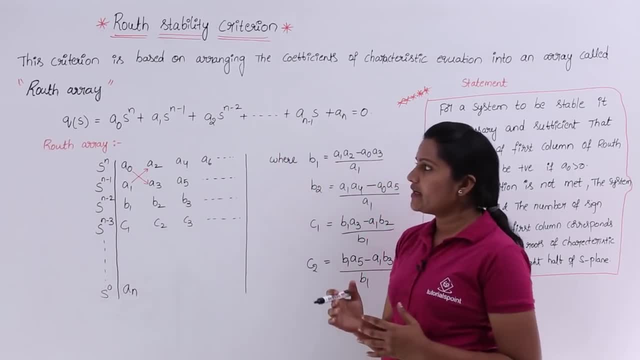 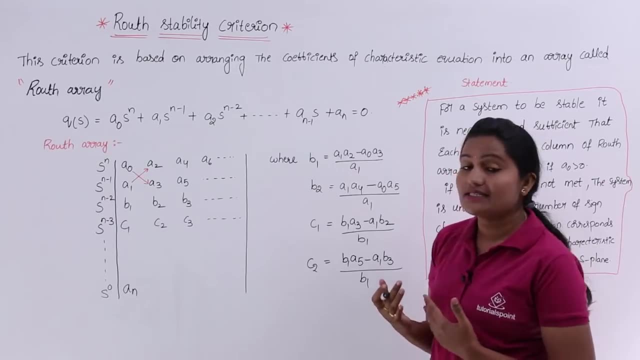 equation. So that is equivalent to a naught s power, n plus a 1 s power, n minus 1 plus a 2 s power, n minus 2 plus so on. a n minus 1 into s plus a n is equivalent to a 1 s power. 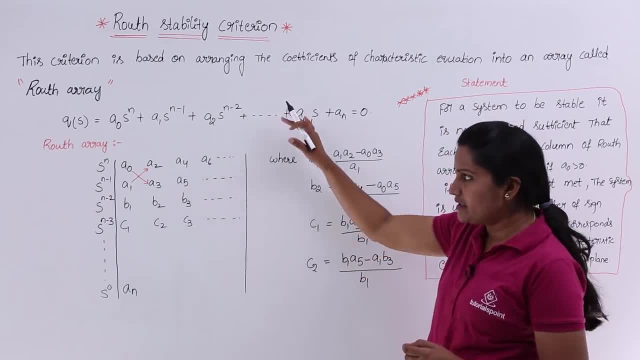 n minus 1 plus a 2 s power n minus 2 plus so on. a n minus 1 into s plus a n is equivalent to 0.. If your characteristic equation is like this, how we need to form the Routh Array means, whatever the coefficients we are having, that. 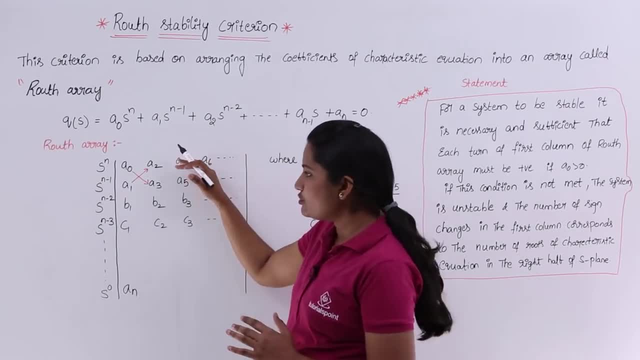 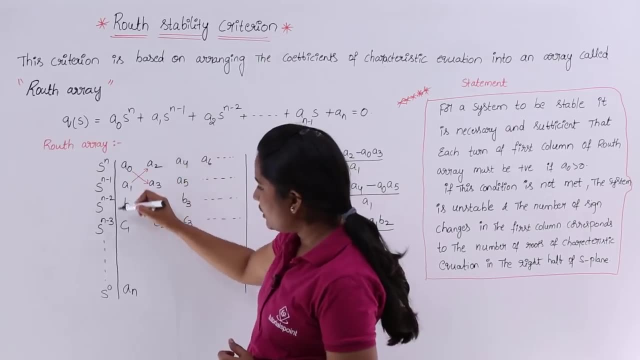 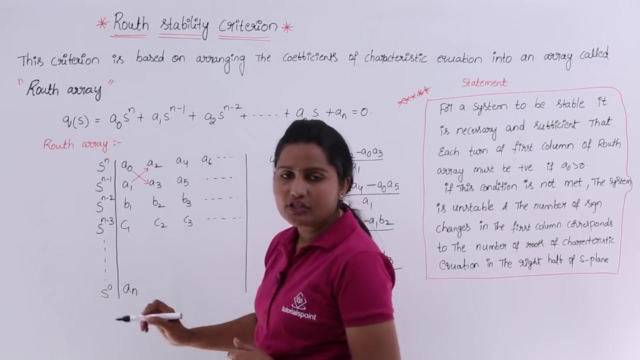 coefficients. we need to arrange in 2 rows, first 2 rows. So we need to arrange the coefficients of our characteristic equation like this. You can see, you need to consider from maximum s power 2, s power 0, that means s power n to s power 0. you need to consider in array. 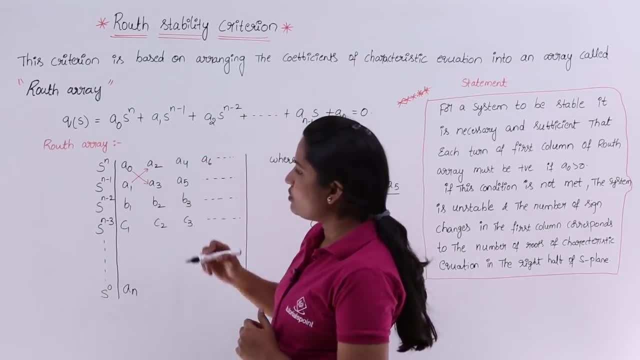 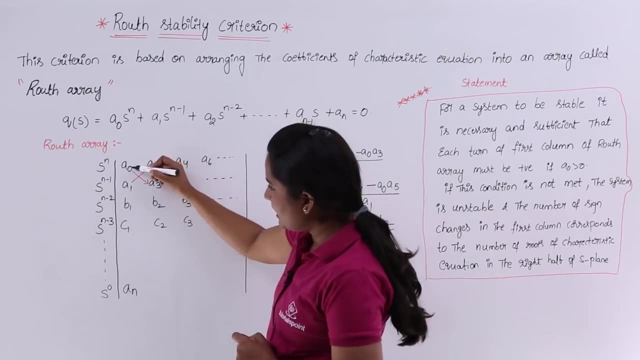 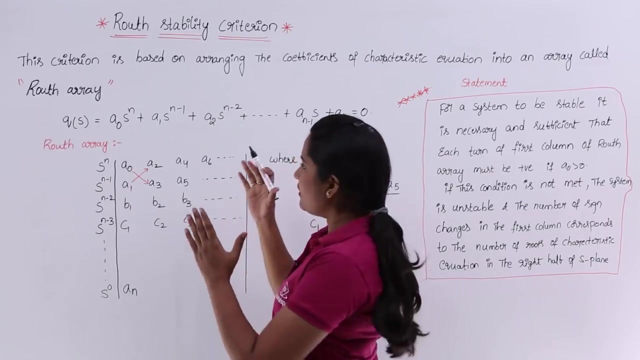 So when you are writing each row, so first 2 rows of this Routh Array can be filled by the coefficients of your characteristic equation. That means you can see a naught- a 1, a 2, a 3, a 4, a 5, a 6- like this. you need to fill the coefficients. So whatever the number, 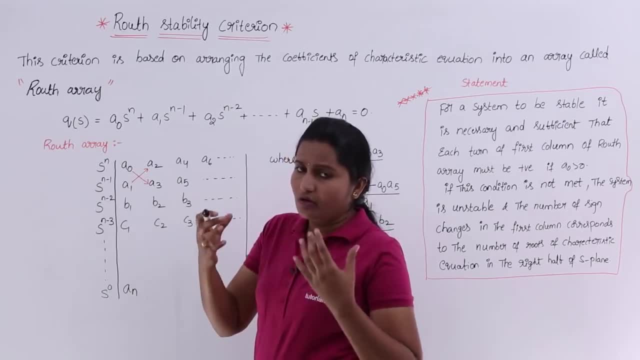 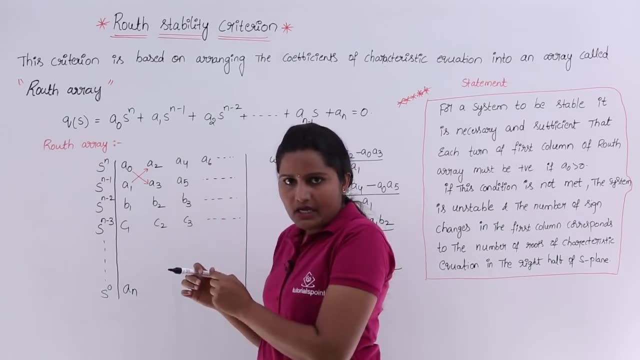 of coefficients. no need of knowledge about how many coefficients we are having. So how many coefficients you are having, that many coefficient that should be there. So you need to place all those coefficients in these 2 columns. That means, for example, if you 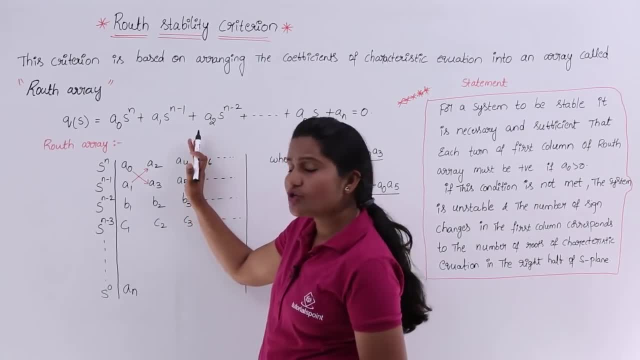 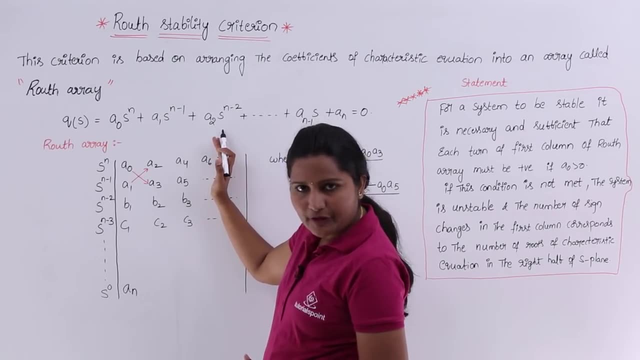 are having up to a 5. only then you can stop this Routh Array up to here. For example, if you are having up to a 6, you just place up to a 6 and you just put 0 here. that is. 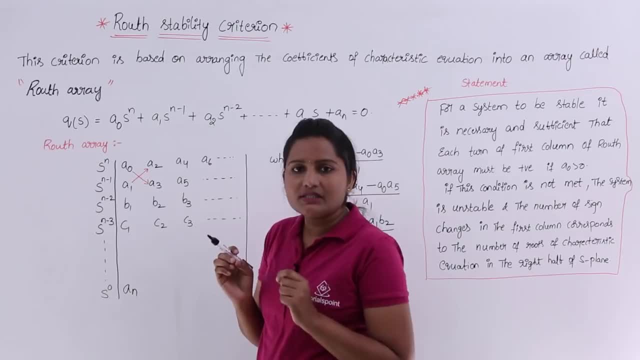 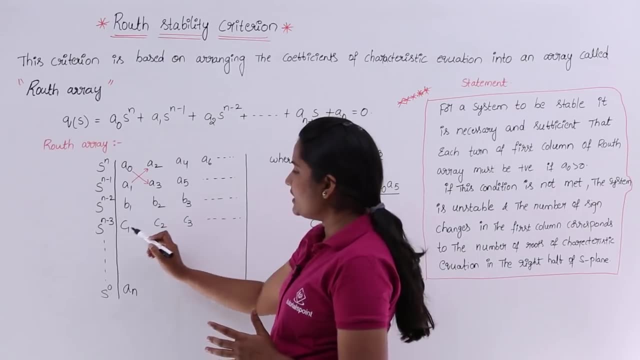 it. So first 2 rows of your Routh Array must include the coefficients of the characteristic equation, And after that So b 1, b 2, b 3, c 1, c 2, c 3, d 1, d 2, d 3, whatever the names you want to put as 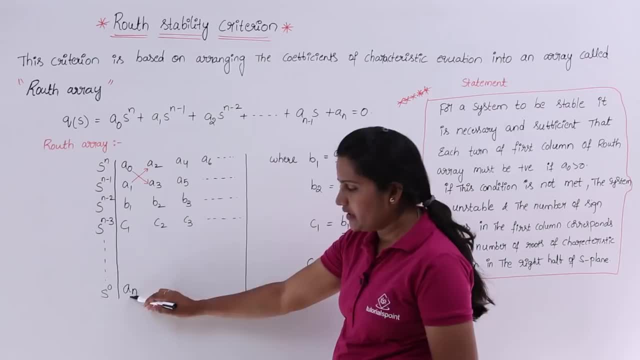 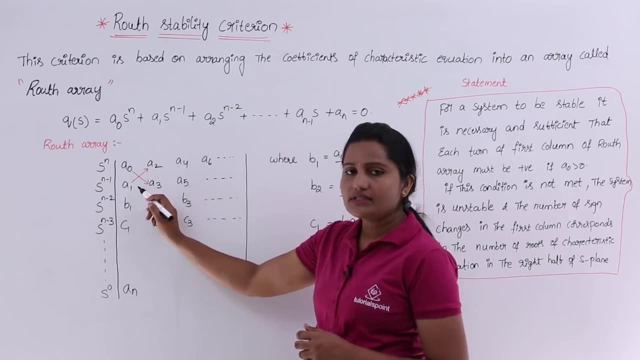 your row names, So that you can put like this: and finally, you are having a n here And now, if you want to get the value here first, 2 rows can be taken from the characteristic equation. Then what is about? third row, fourth row or what may be? the next rows are there? 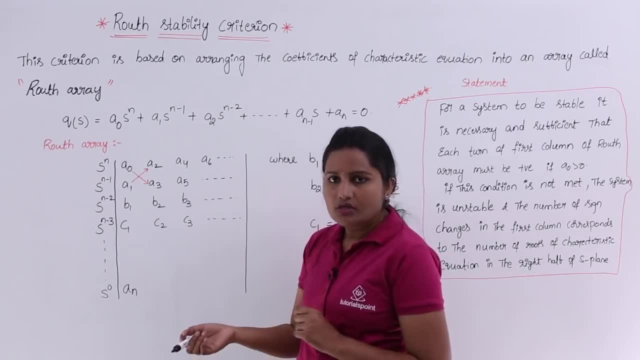 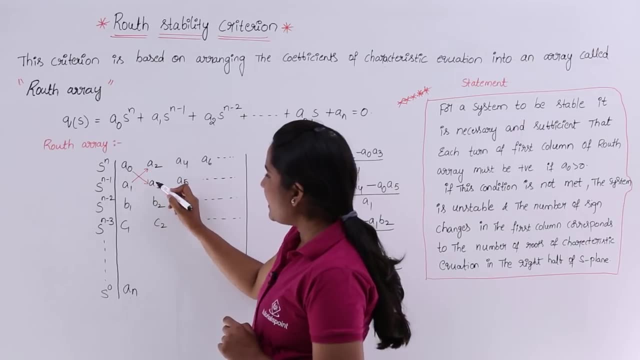 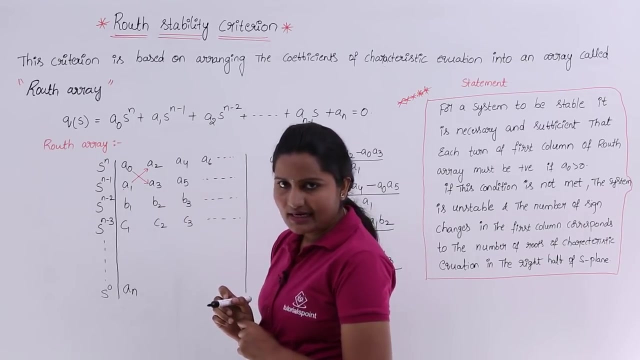 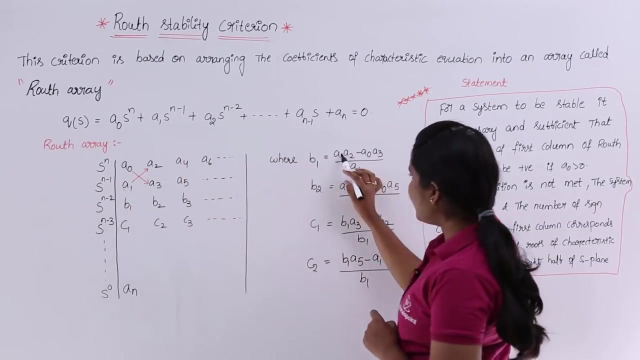 that next rows can be calculated from the characteristic equation. So that is what we mean by a 1, a 2 can be calculated from the characteristic equation. they just let you know a comma semicolon. So that means, for example, if you want to calculate b 1, then a 1, a 2 minus a naught. a 3 divided by a 1, we will take. So, whatever the value above, a 1 is there that you just consider as the reference: a 1, a 2 minus a naught, a 3 divided by a 1.. So you can see a 1 a 2, a naught a 3 divided. by a 1.. So like that you can see, if you want to, for indicating mtt by a 1, a 0. a 1 may not be a 1 dot at a kétat b 1 tube is x, n, b. So here leaders, and cortar y is boils are. 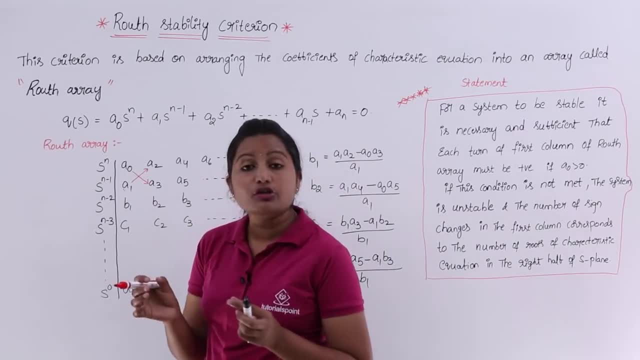 alsom they should be. Thank you also, haveULLA Forahl aha 저. Okay, So this will define the integer number in the sexy limit which you set. that animation is which refers to the frame for b 2. if you want to calculate b 2 value and if you want to place b 2 value there. 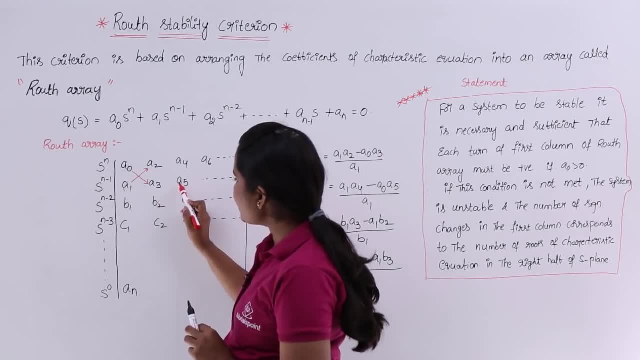 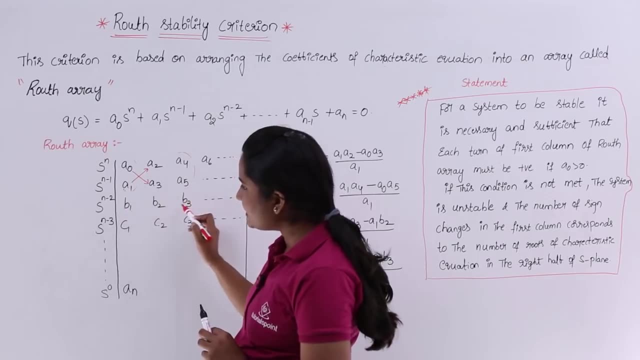 then. so here, whatever the crash value is there, so that values, you just consider and starting values, always to get the third row, always to get the third row first, two column elements, that means a naught, a, 1 are must, and to get b 1, so this cross row is combined with this. 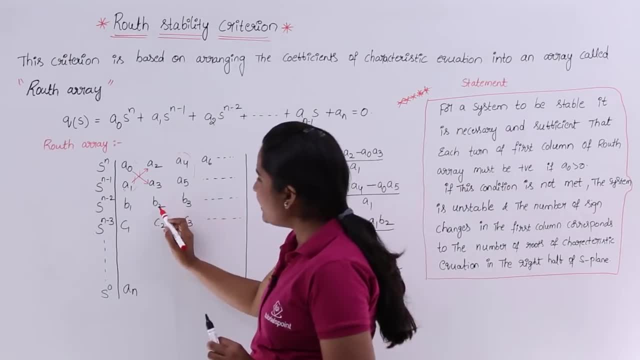 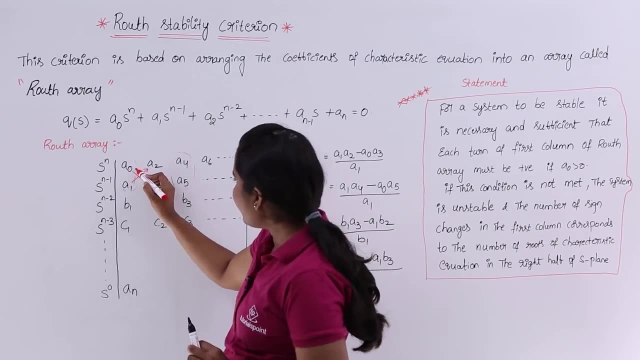 row and we are getting this equation to get b 2. first, two elements and this cross elements. these two are needed to get b 2, like a naught a 5, and here a a 1, a 4 minus a naught a 5. 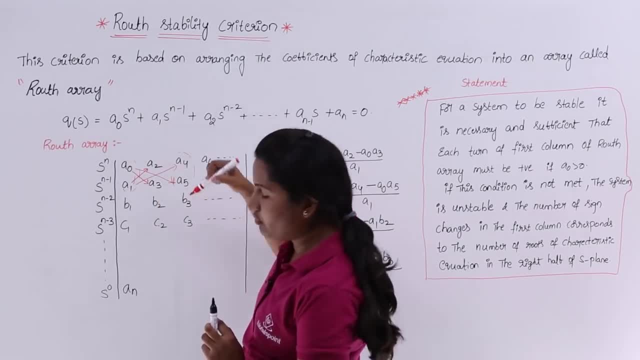 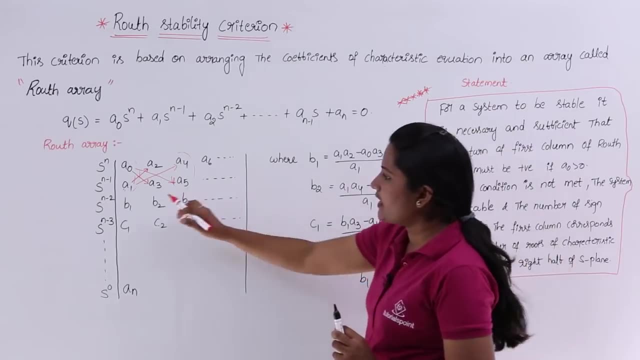 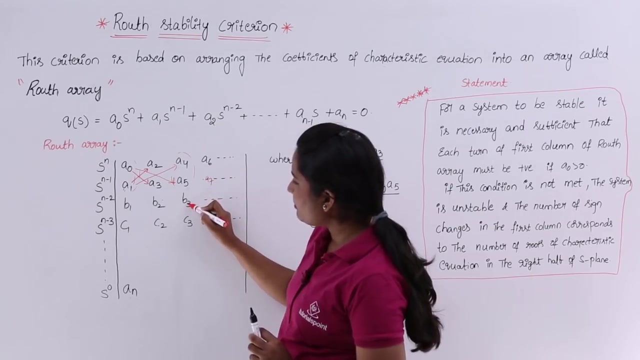 first down to top and top to down. So a 1 a 4 minus a naught a 5. so a 1 a 4 minus a naught a 5 divided by a 1. for example, if you want b 3, so here you may have a 7, right. so if you want b 3, so a 1 a 6, a naught a 7. 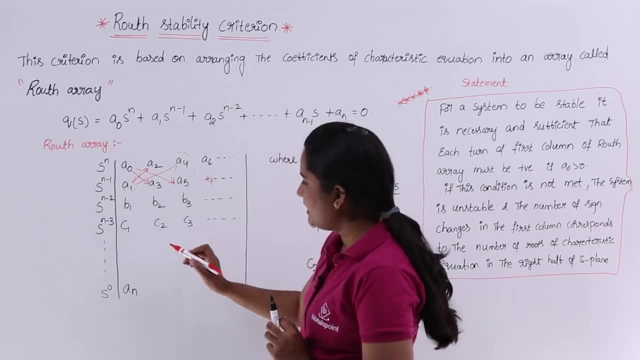 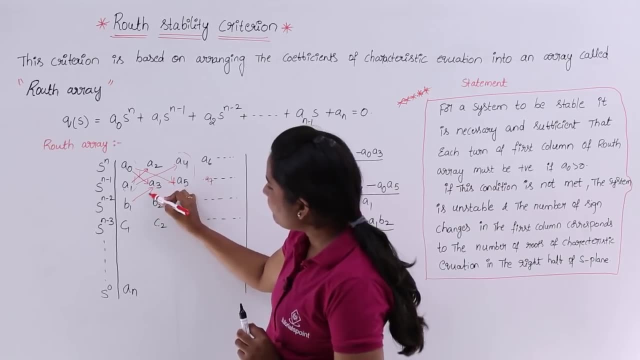 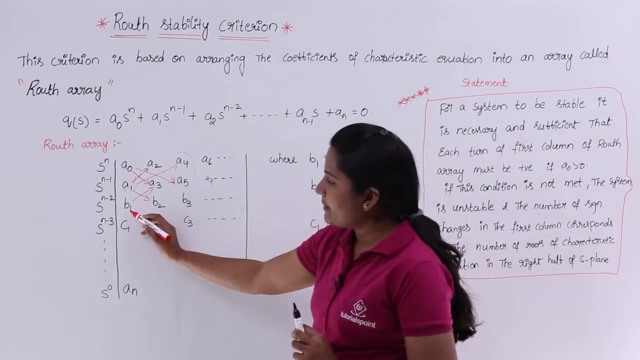 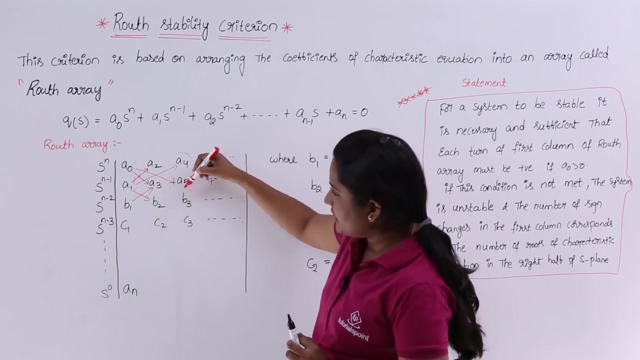 divided by a 1 will take. So here, similarly, if you want c 1, so if you want c 1, so you can take like this: b 1 a 3, a 1, b 2.. b 1 a 3 minus a 1. b 2 divided by b 1. if you want c 2, then b 1 a 5, a 1 b 3. b 1 a 5 minus. 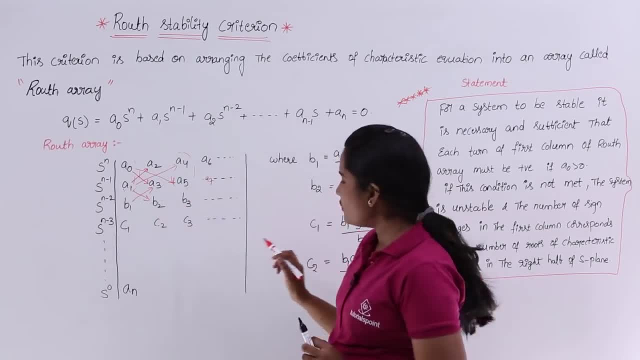 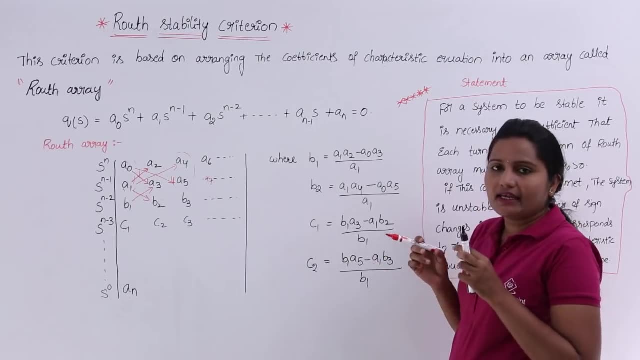 a 1, b 3 divided by b 1 only. So like this, you can write the values in the route array. first two rows must be taken from the characteristic equation, and after that, the next row. you can write the values in the row array. 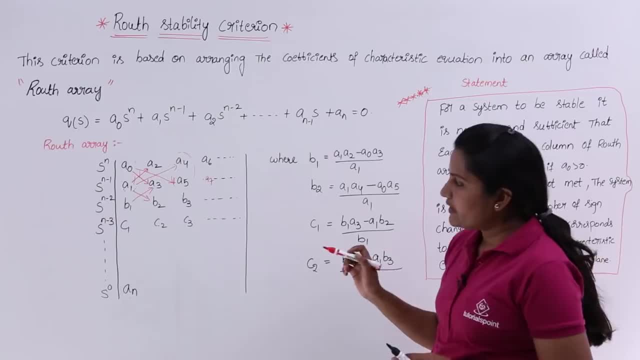 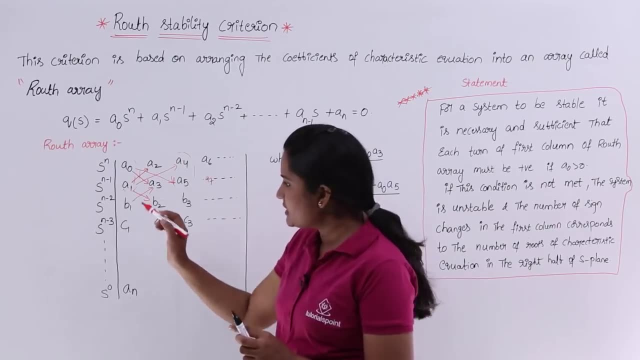 So the first rows can be calculated from the previous rows like this: first you need to consider like this: So a 1, a 2, a naught a 3, minus in between, minus divided by a 1. if you want, b 2, so this: 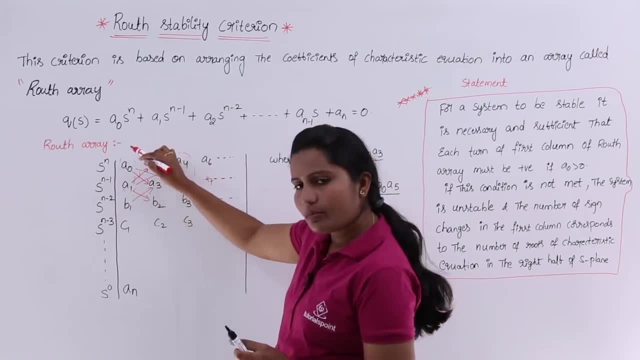 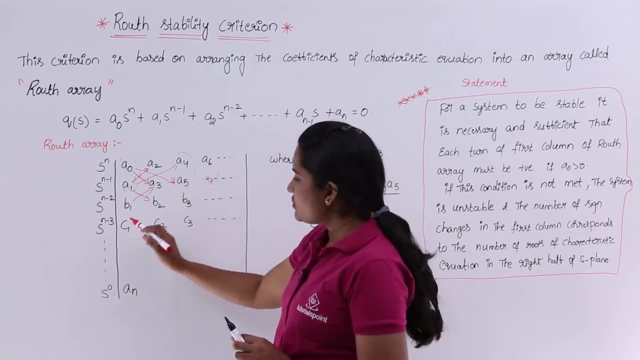 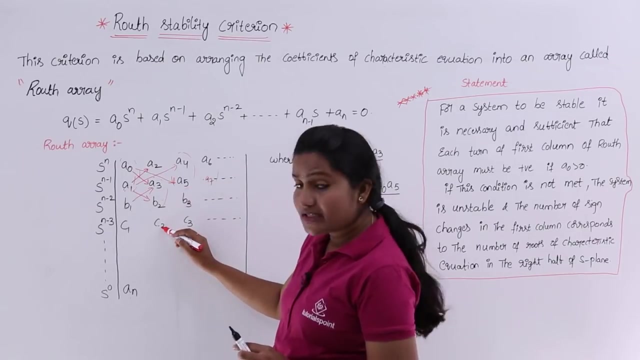 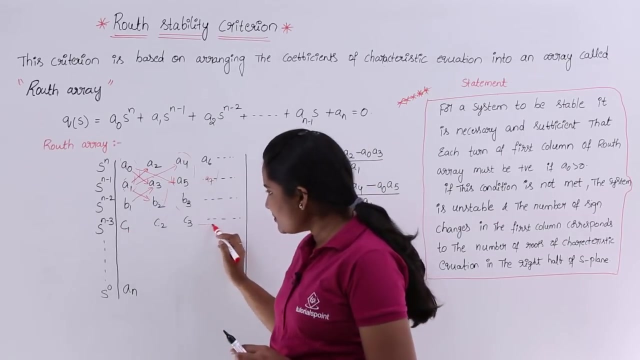 combination, this combination, if you want b 3, first combination is always must. So this combination, with this combination, you need to consider to get b 3. So here, for example, c 1. First they calculate b 2 and you colostrum. 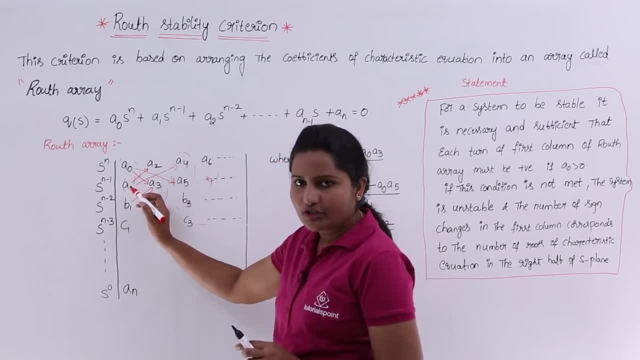 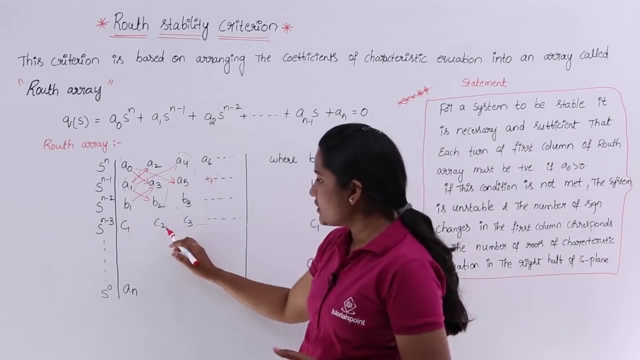 like this: First to get c 2 cross combination: first combination: cross combination means해웰 unleash. you need to consider. So to get this row divided by b: 1, need to consider. to get this row divided by a: 1, you need to consider. 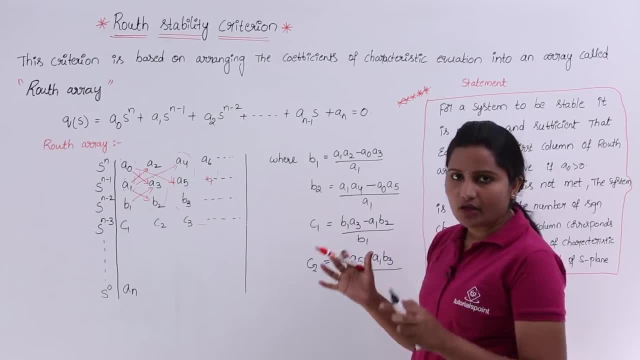 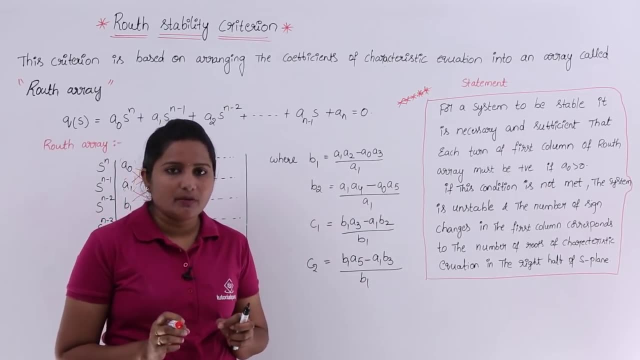 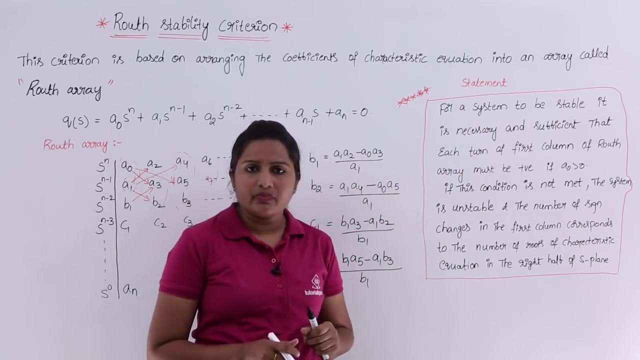 you can see, to get b 1, b 2 or b 3, anything divided by a 1 will be there. to get c 1, c in routh array. and very important point: after writing routh array you need to observe very important point, that is routh hertz criterion statement. so for a system to be stable, for 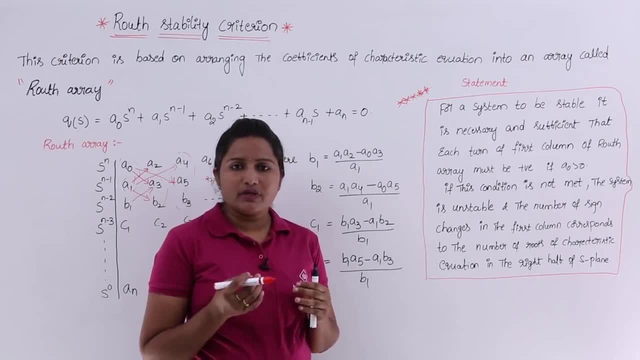 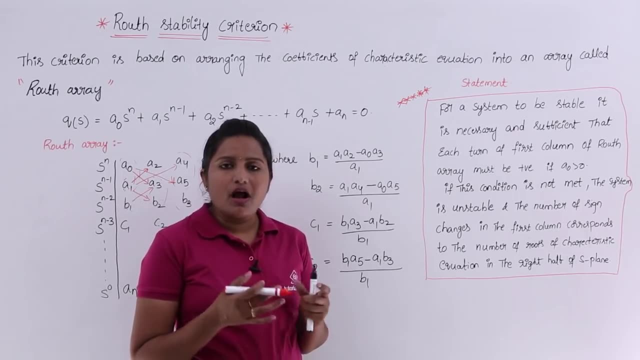 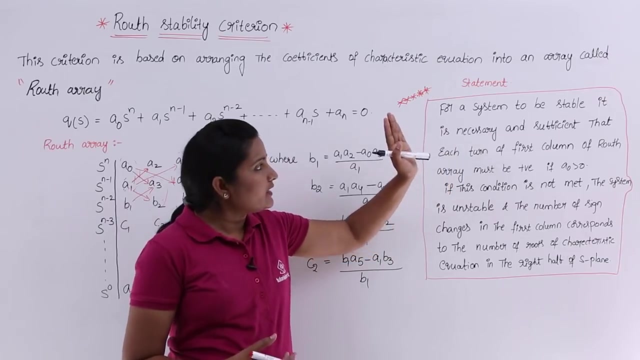 which purpose we are doing. this criterion means to estimate the stability of the system. we are doing routh hertz criterion, so routh array, we are making routh array. so, after making this routh array, what we need to see. so this is the statement for routh hertz criterion and here for a system to 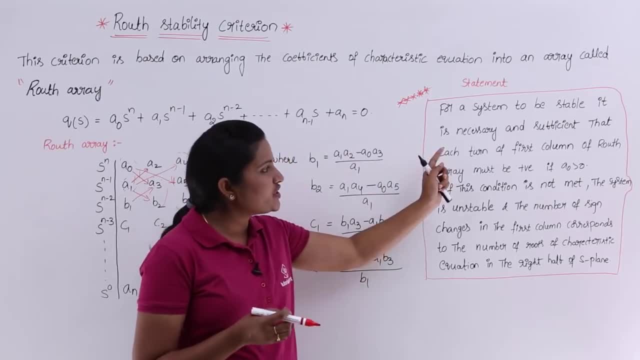 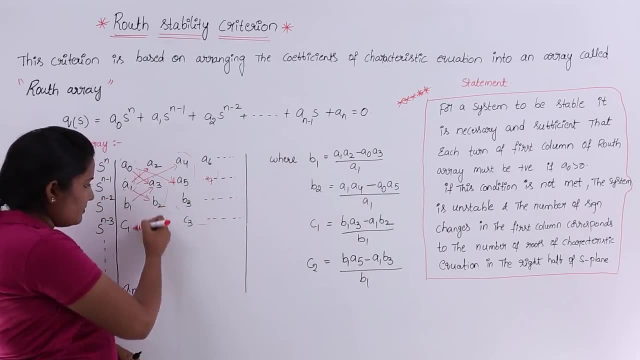 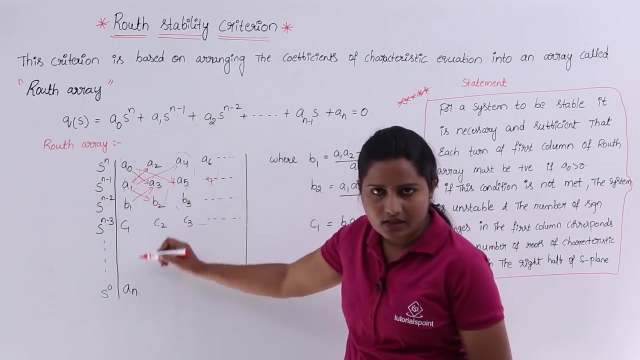 be stable. it is very necessary and sufficient condition that each turn of first column, that means this column, each turn of first column, is this column. after making whole routh array, we need to observe the first column, each turn of first column, and here that must be positive. 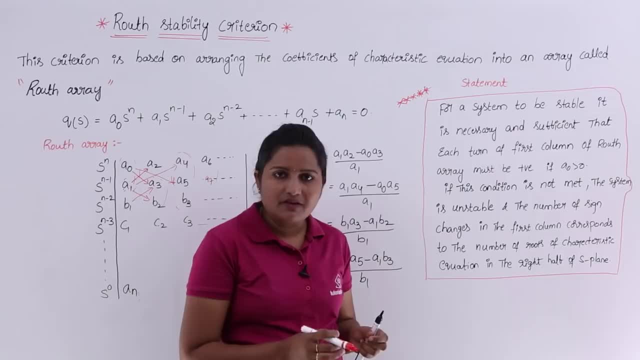 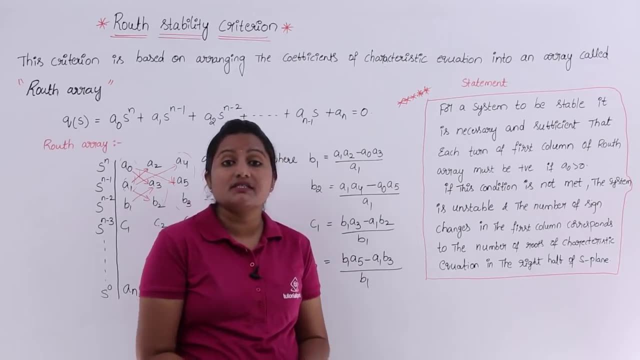 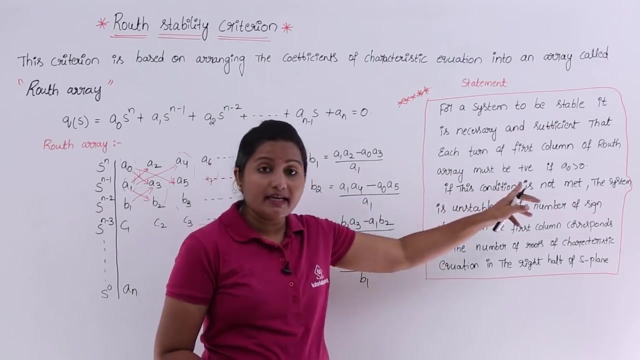 after making routh array. this is very sufficient condition that each turn of first column must be positive to say the system is stable. if that first column is not positive, if you observe any negative sign, that means if you violated, if you are not meting that condition, then you can say the system is unstable. 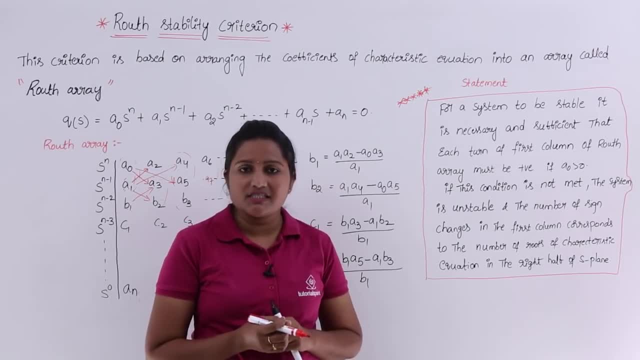 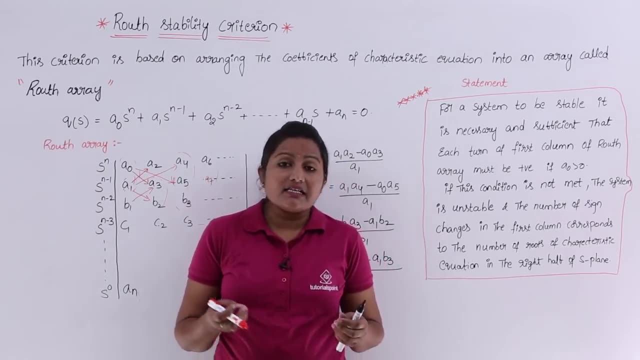 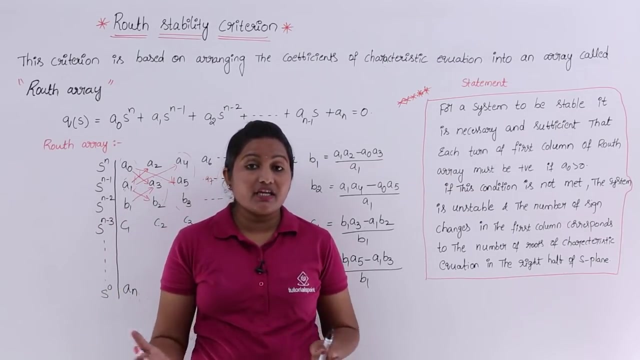 system and the number of sign changes will indicates the number of poles shifted to right. when we will say a system is unstable system means whenever any pole shifted to right half of s plane, then we can say the system is unstable system. this number of sign changes, for example, if you are 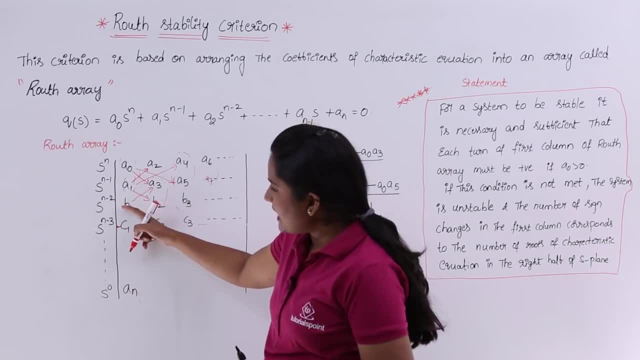 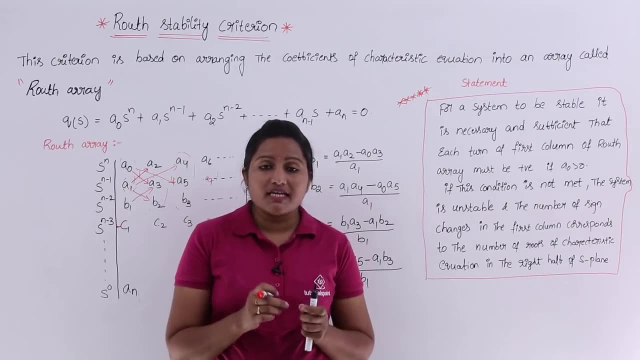 having minus here. so the sign changes positive to negative and then negative to positive. so two sign changes are there. so that number of sign changes will indicate the number of poles moved from left to right to make the system unstable. so this is very important statement. once again, i am going. 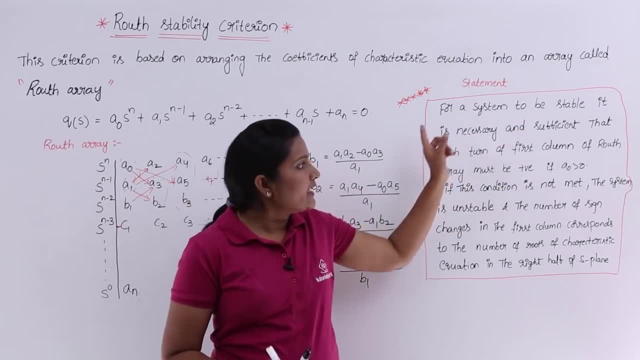 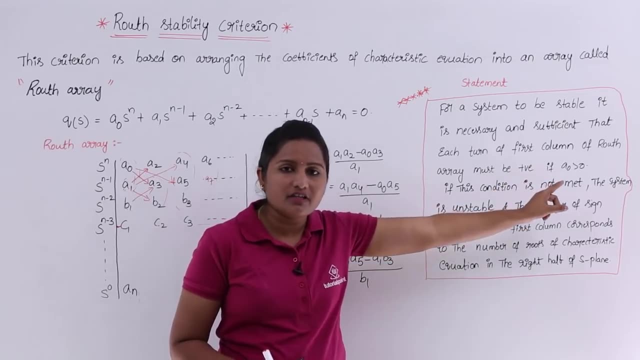 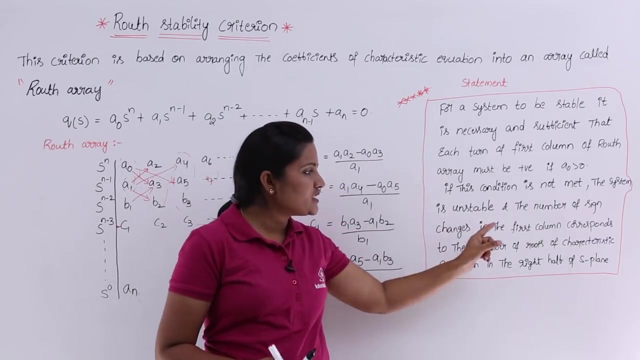 to repeat the statement that is, for a system to be stable, it is necessary and sufficient that each turn of first column of routh array must be positive if a not greater than zero. if this condition is not met, the system is unstable and the number of sign changes. in the first.